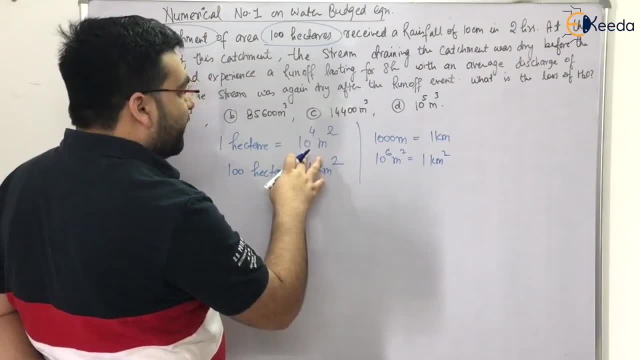 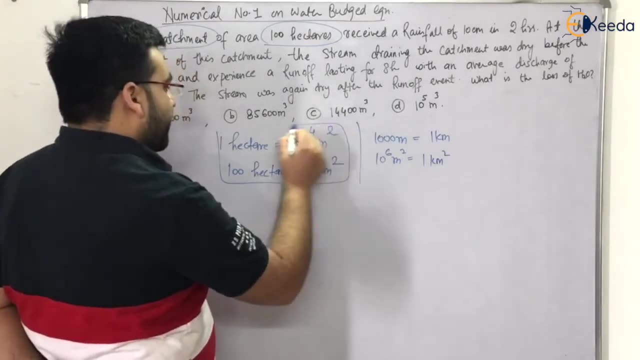 just you can just put it like this: divided with 10 raised to power 6, right, so you will be getting 10 raised to power 6 square 1 minus 2, that is, 100 hectares, is 1 kilometer square, right. just remember this and you will. 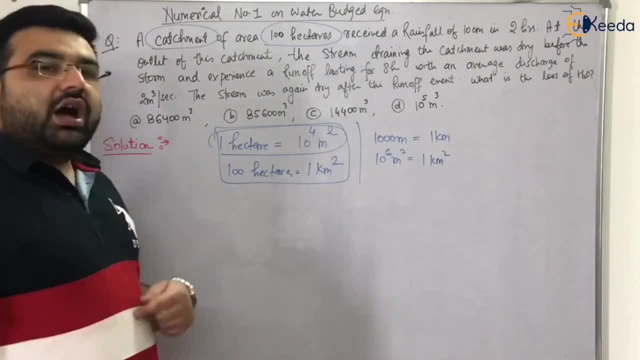 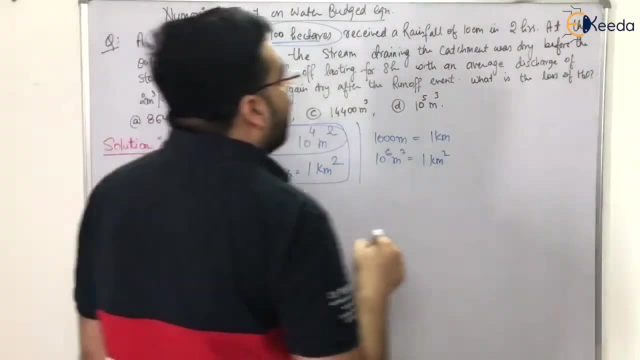 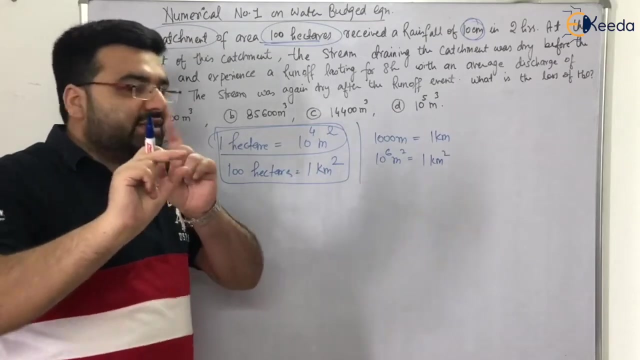 get the other holes right. so hectare is a very common unit in hydrology as well as in irrigation clear now, a catchment of 100 hectares received a rainfall of 10 centimeter. 10 centimeter is the rainfall. it means that the depth of the rainfall is given to you. the depth of the rainfall is given. 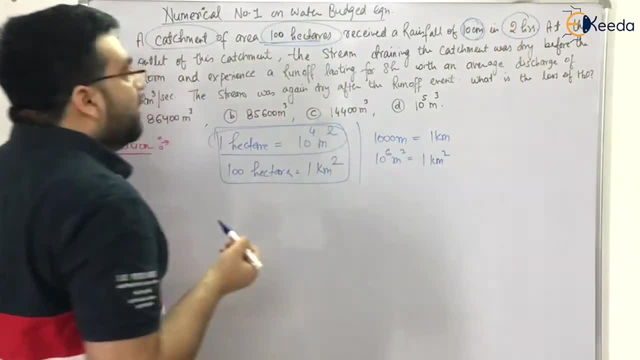 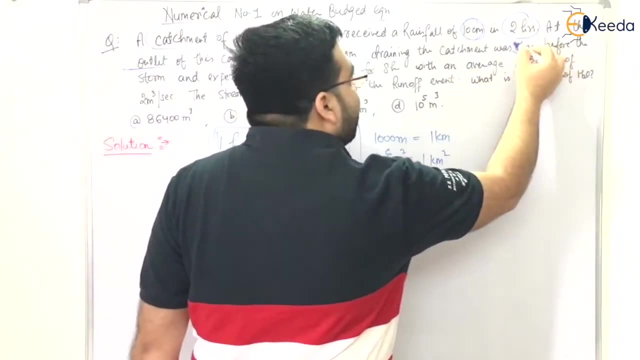 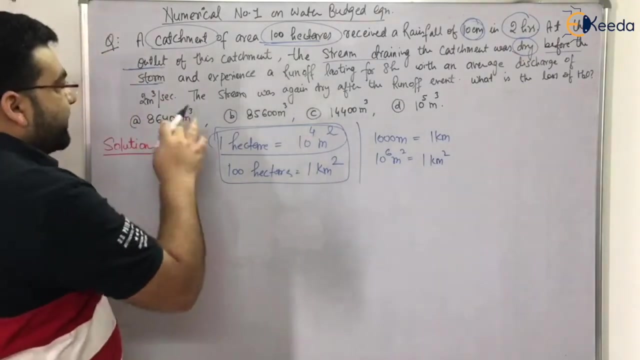 to you right in two hours. so time frame is also given. at the outlet now, at the outlet of this catchment, the stream draining, the catchment was dry, dry before the storm. so when the storm came before it was dry, the stream was dry right and experience a runoff lasting for eight hours. so 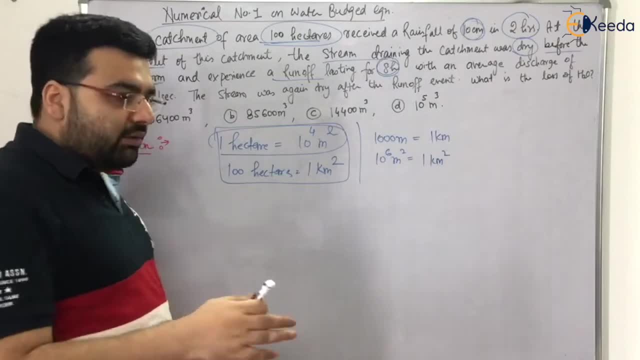 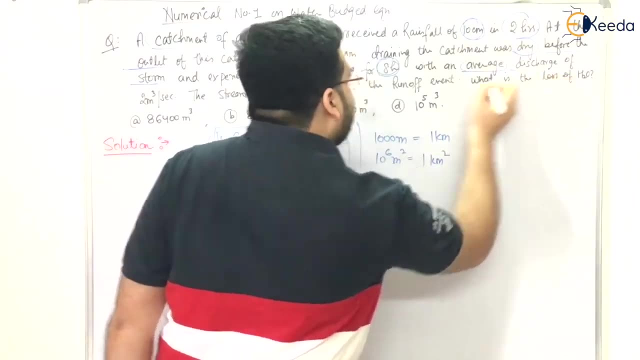 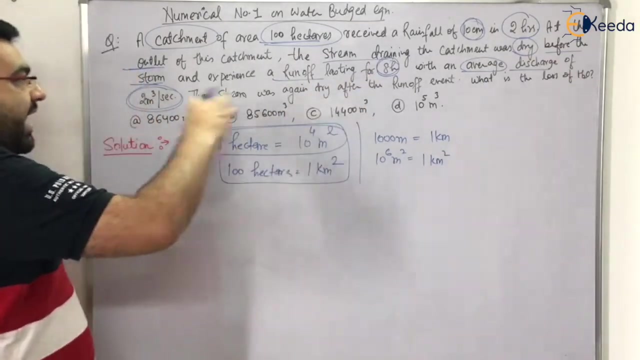 now, after the precipitation has come, after the rainfall has come, the stream it has. you can say it has lasted for eight hours, right with an average discharge. average discharge is given to me as two meter cube per second. now i can determine the volume also because time is given to me for how much time. the average, this is the average discharge. 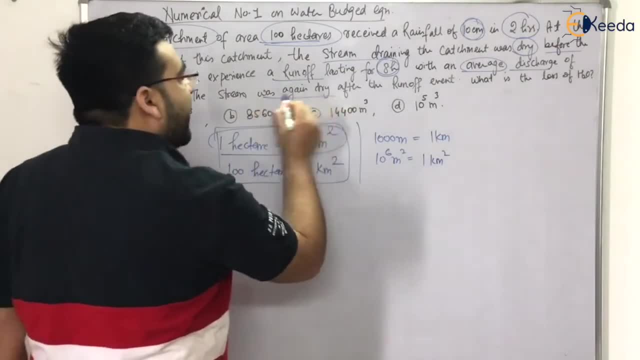 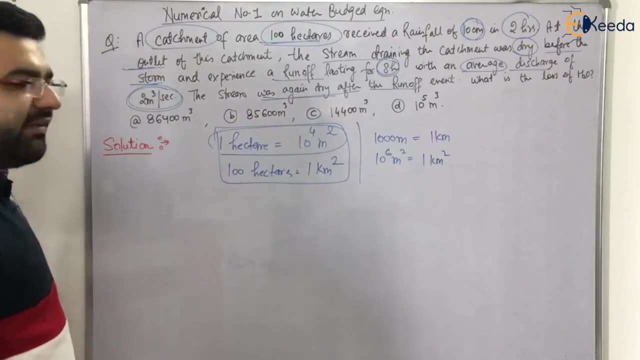 i can determine the volume also. right, the stream was again dry. now it is again dry after the runoff. right, it is again dry. what is the loss of water? this four options are given. so it's a very easy question. just apply the water budget equation, you will get the answer. so let us apply the water. 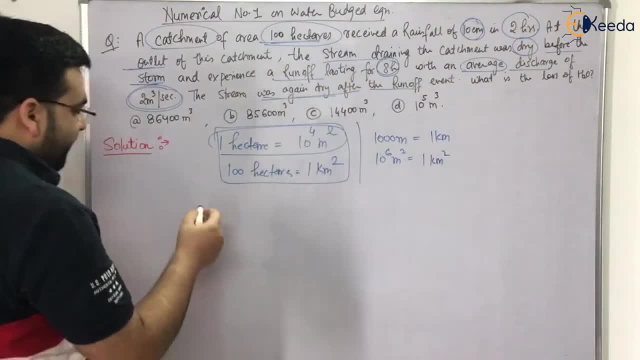 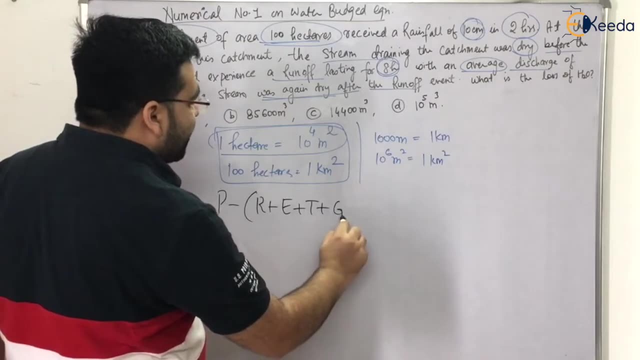 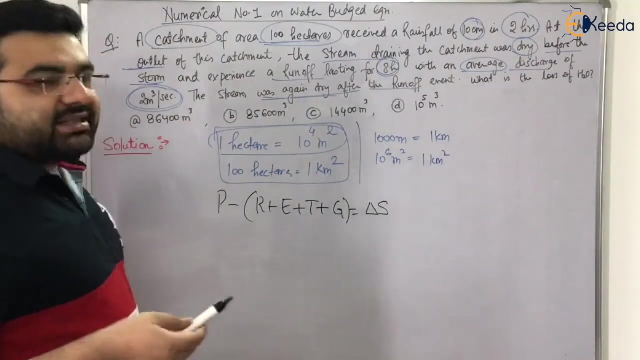 budget equation, we have to calculate the losses. so i told you that the precipitation minus runoff, plus evaporation, plus transpiration, plus groundwater will give you storage. how much the storage is right? or you can say that the inflow minus outflow will give you storage right. 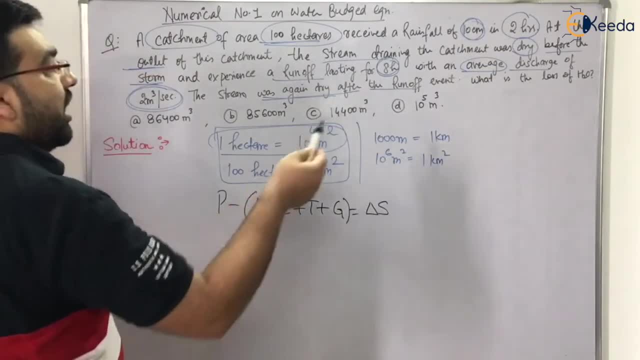 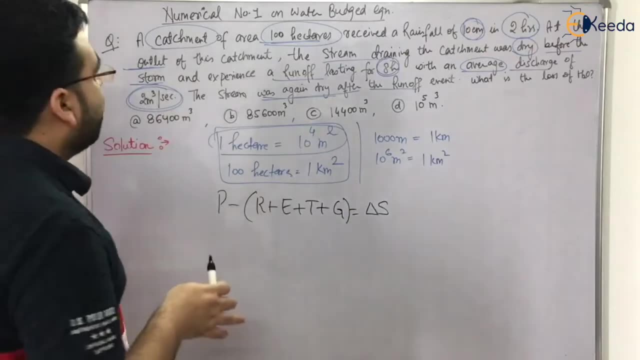 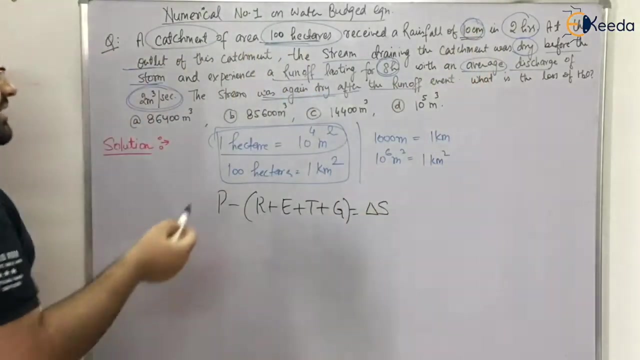 so let us see that in this equation, uh, catchment is given to you. now what will the inflow? so, inflow will be the precipitation which has occurred, right? so over a, over an area of 100 hectares, is 10 centimeter. the rainfall is 10 centimeter. so let me first of all calculate the volume, right? 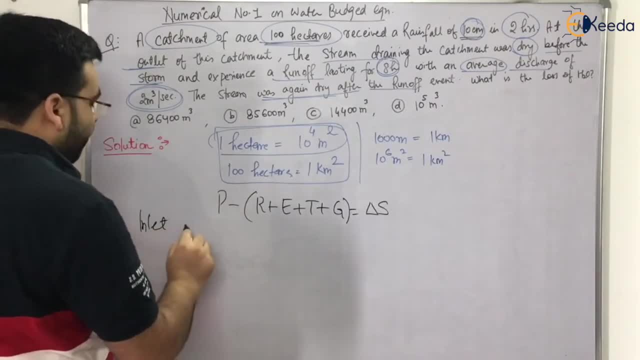 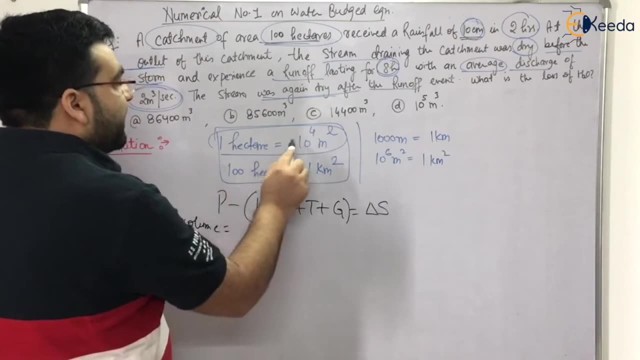 so inlet volume. so inlet or inflow volume will be equal to how much hectare is 100 hectares? i know that one hectare is 10 is for 4 meter square. so 100 hectare will be equal to 10 is for 6 meter. 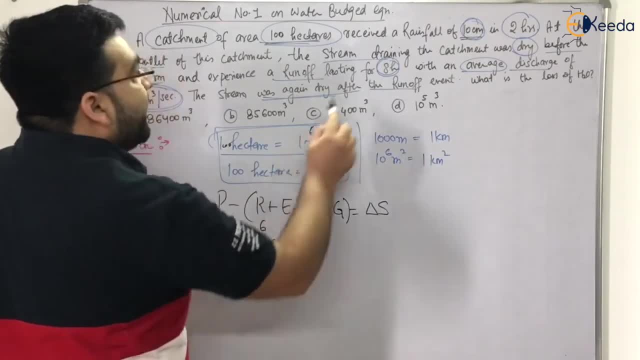 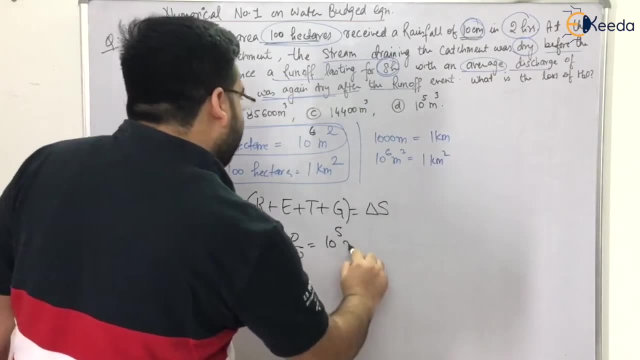 square right. so 10 is for 6 meter square. into 10 centimeter. let me convert it in meter so it will be equal to 10 raised to the power. 5 meter cube is the inlet. 10 square 5 meter cube is the inlet now. 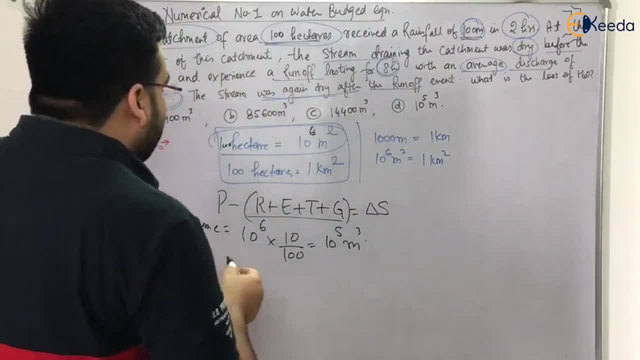 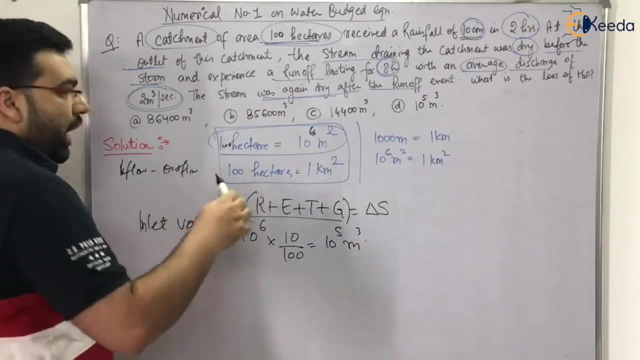 let me calculate the outlet also. so outlet will be equal to: in: inflow minus outflow, right, inflow minus outflow. so how much is outflow, outflow which is going away from the stream, right? how much, uh, it is going away from the stream. so 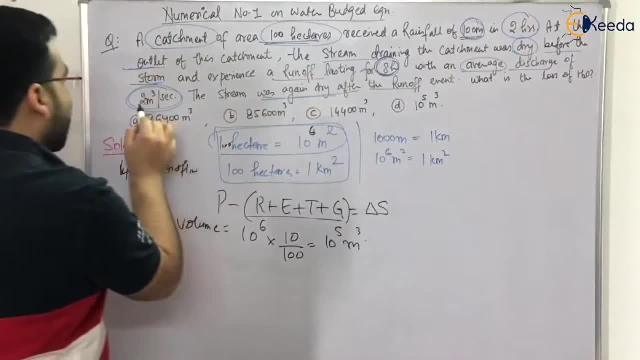 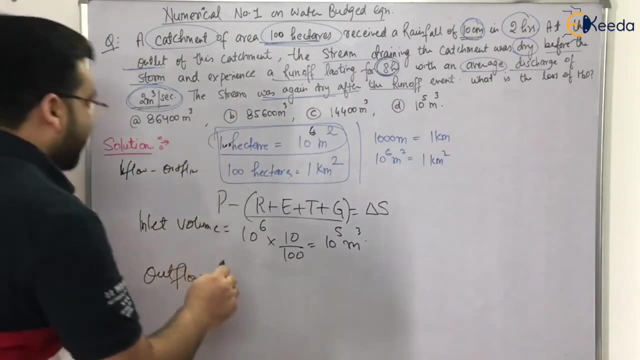 a runoff lasting for eight hours with an average discharge of two meter cube per second. now let me calculate outflow also outflow. outflow will be equal to the discharge is given to you- two meter cube per second. into time. now time will be in seconds. so eight hours is given to you, so eight. 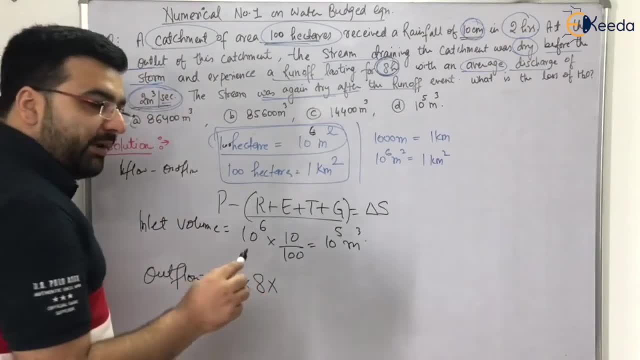 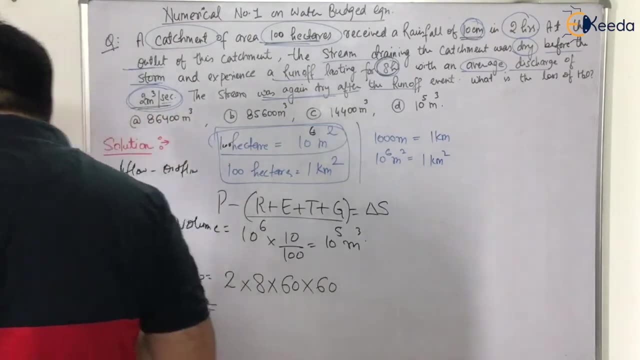 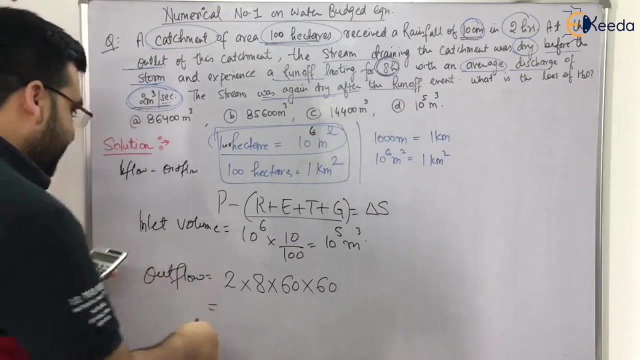 hours. clear now how many, uh, how many minutes it has 60 minutes and how many seconds per minute has 60 seconds. so this will be equal to. let me calculate how much will it be. so it will be equal to eight into two, into three, six double zero. it comes out to be five, seven, six double zero. it comes. 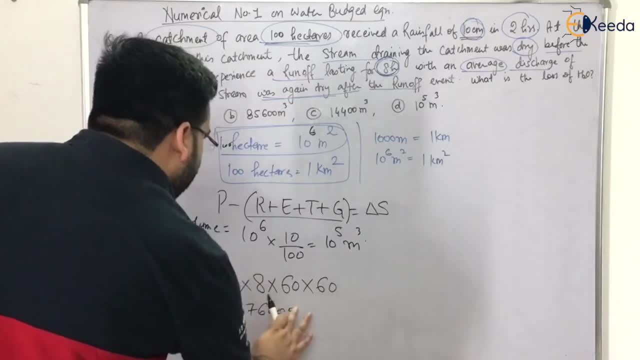 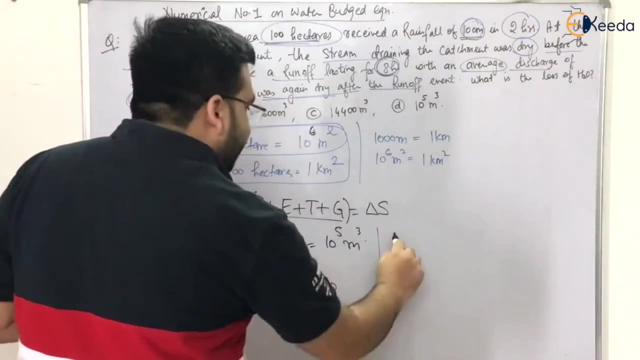 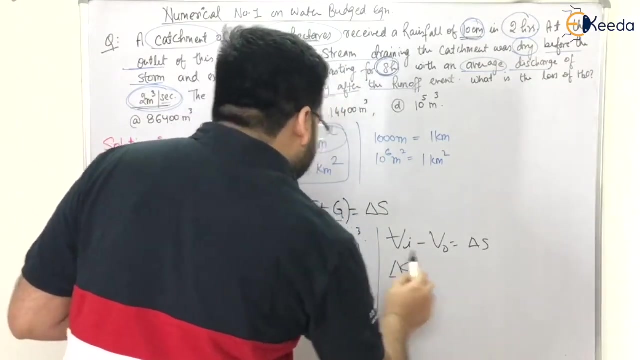 out to be five, seven, six, double zero meter cube. right, so this is the discharge. now let me subtract these two. that is, inflow minus outflow will be equal to delta storage and delta storage will be the losses. so it will be equal to storage. can be in the form different depressions. it can be in the 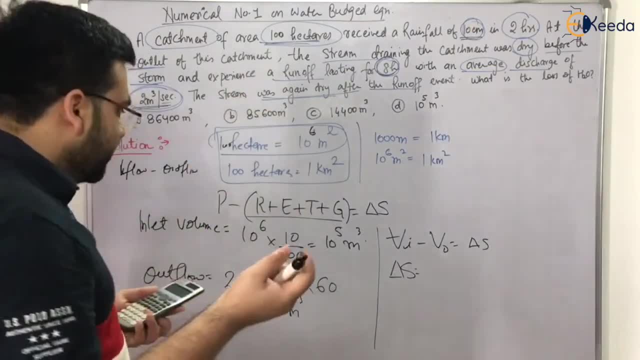 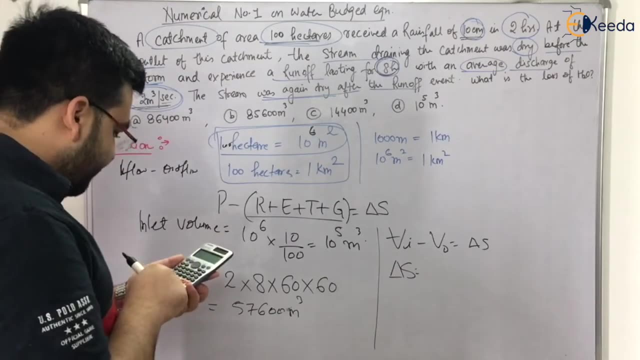 form of, you can say, or plants also, there can be some storage. so that is the losses, right. so it will be equal to 10 raised to power. five minus five, seven, six, double zero. it comes out to be four to four double zero. it comes out to be: